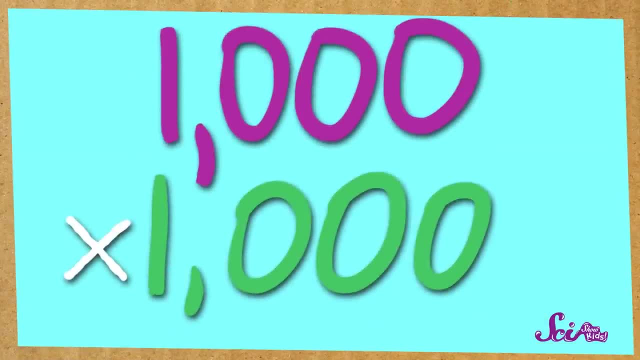 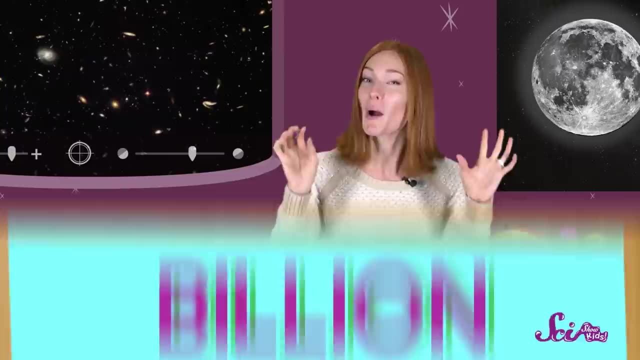 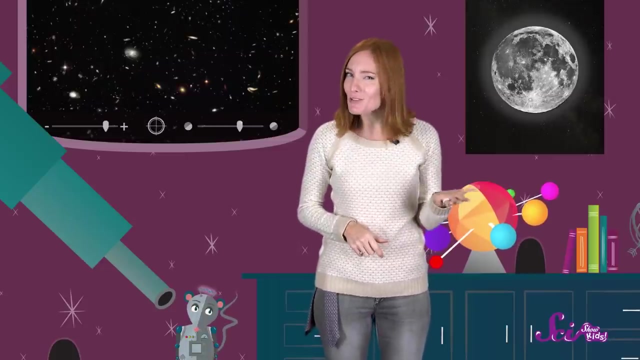 A thousand looks like this: And if you take a thousand and multiply it by a thousand… And multiply it by a thousand again, That number is a billion, And there are billions of stars just in the Milky Way alone. In fact, there are so many stars in the Milky Way that we still don't know exactly how. 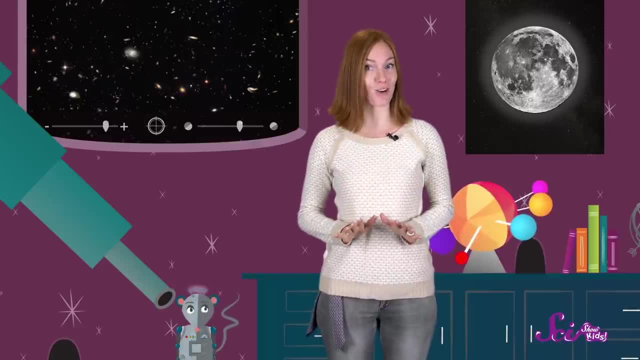 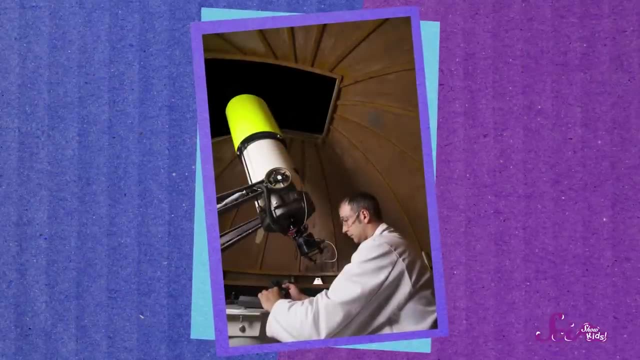 many there are, But scientists think that many of the other stars in our galaxy probably have planets of their own. And the Milky Way isn't the only galaxy. Astronomers who study deep distant space have found other galaxies too, More than you could count. 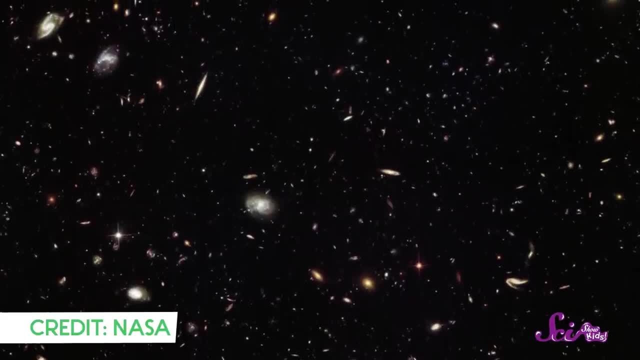 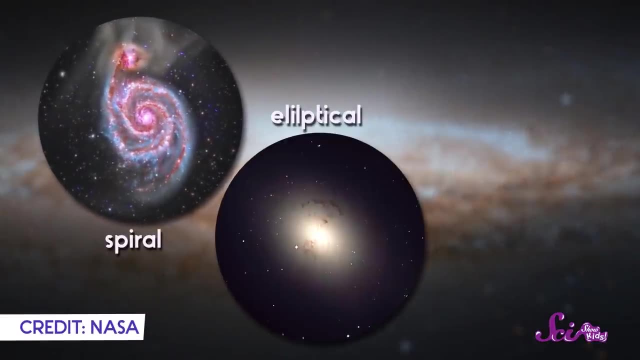 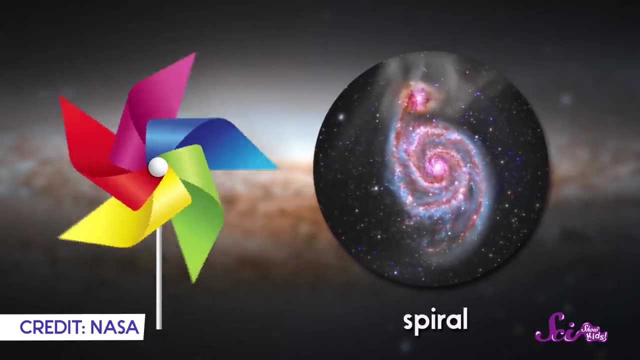 To organize and study all of these galaxies, astronomers usually group them into three main types, depending on their shape. There are spiral galaxies, elliptical galaxies and irregular galaxies. Spiral galaxies are in the shape of a pinwheel. They have that shape because stars in a spiral galaxy are clumped into lines that curl outward. 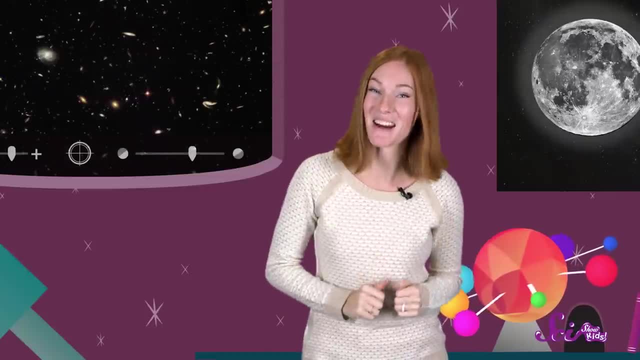 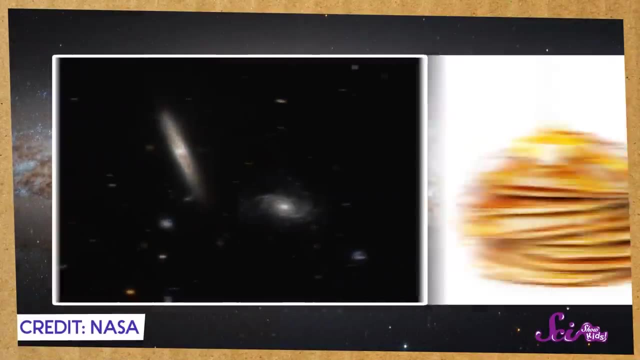 These lines are called spiral arms, And the galaxy that you and I are in right now, the Milky Way galaxy, is a spiral galaxy. The Milky Way is a spiral galaxy. Now some spiral galaxies are just flat like a pancake. 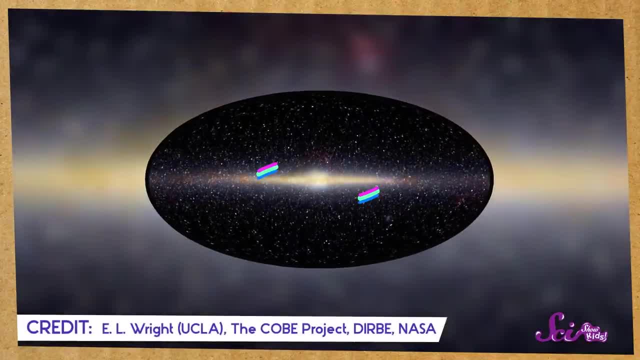 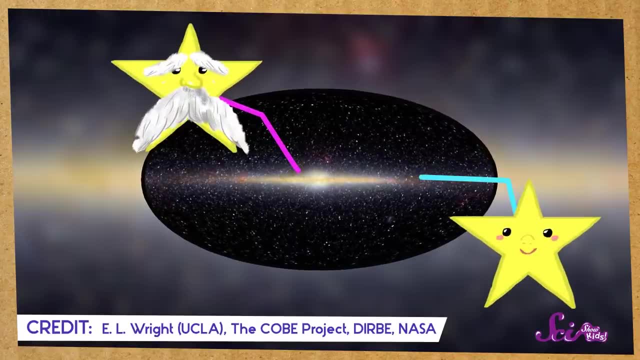 But other spirals, including our own, Milky Way, have a large bulge in the middle that's made up of a big bunch of stars. The stars in the bulge are usually older stars, while younger stars are often found on the outer spiral arms of the galaxy. 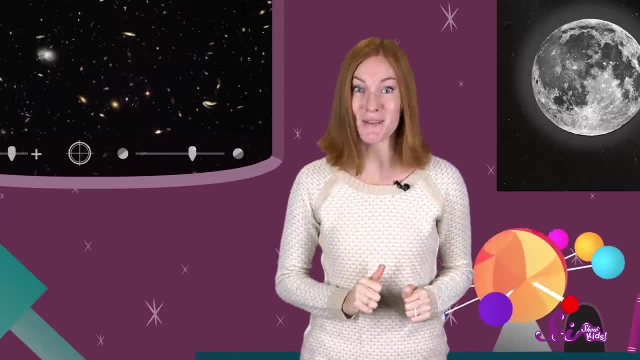 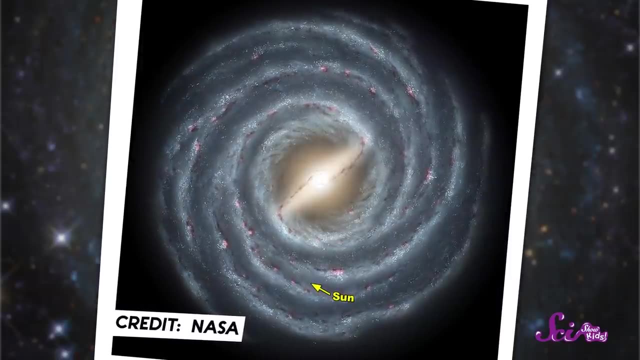 Astronomers even know where our star, the Sun, is in the Milky Way. If you were way, way out in space floating above our galaxy and looked down at it, you'd find the Sun right about here, Near the middle of one of the spiral arms. 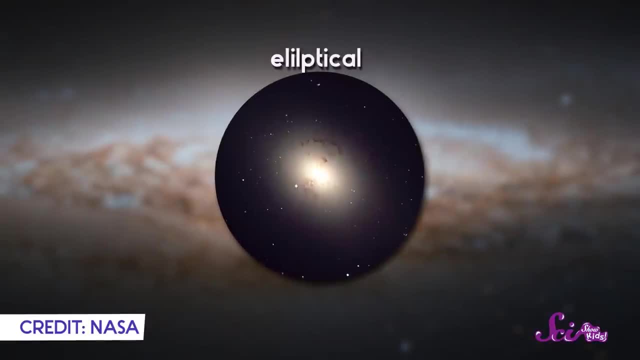 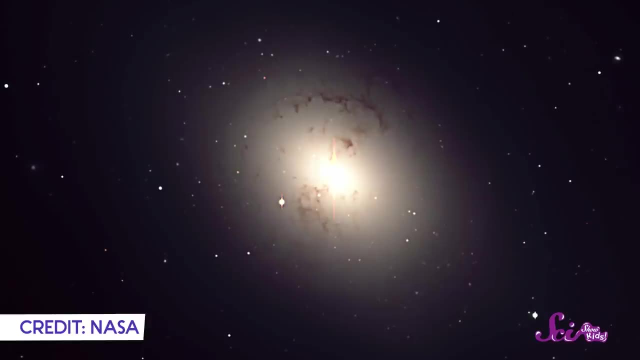 Now another common kind of galaxy is called an elliptical galaxy. Elliptical galaxies are shaped like an ellipse or an egg shape And instead of being flat with a bulge in the middle, these galaxies are all bulge. They tend to have mostly older stars in them, and stars in an elliptical galaxy are really. 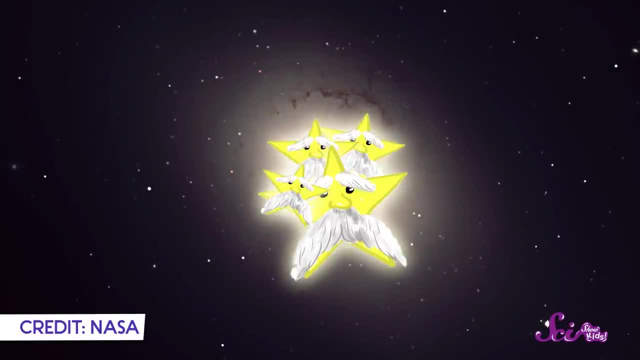 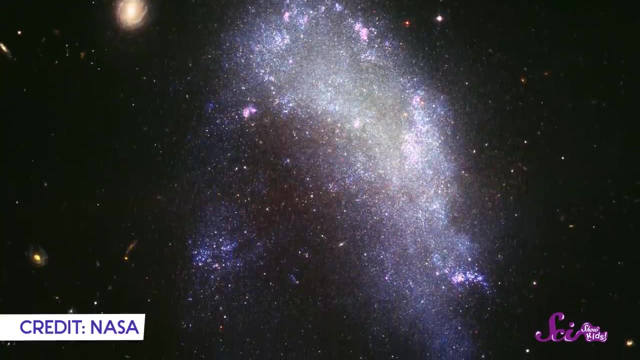 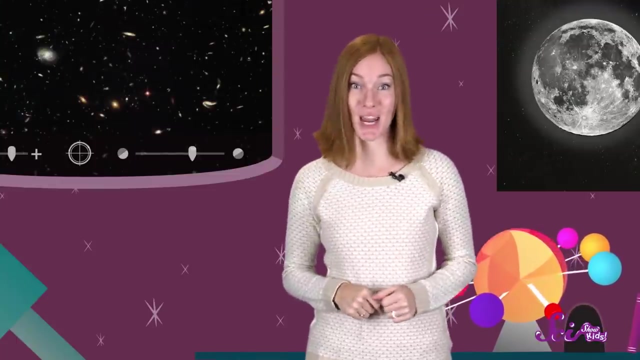 close together, which makes the middle of the galaxy look like one giant bright star. The last common type of galaxy is an irregular galaxy. Irregular means not regular, And these kinds of galaxies don't have a definite regular shape. Instead, these clusters of stars can take all kinds of different shapes, like this: